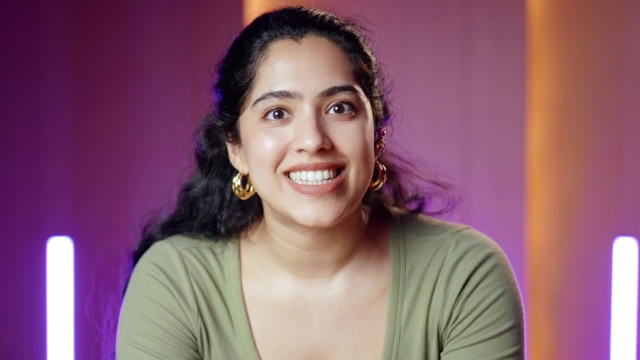 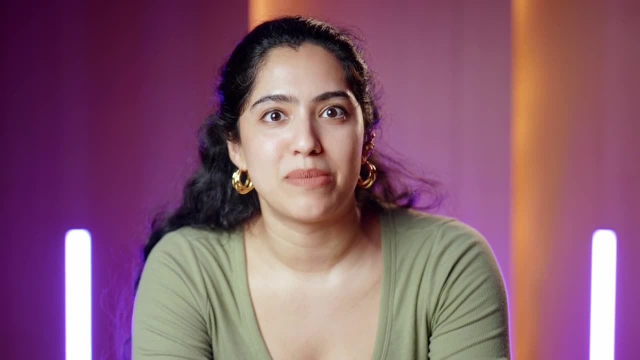 is simple if data doesn't change much. Unfortunately, that's not the case with most modern systems. So how do write requests cascade across multiple identical databases with timeliness and consistency? There are a few strategies to choose from, though as always, there are trade-offs. 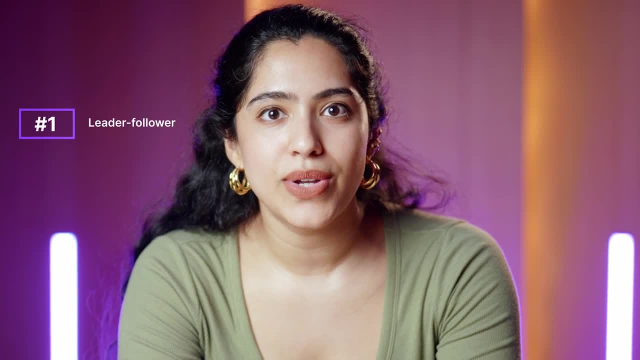 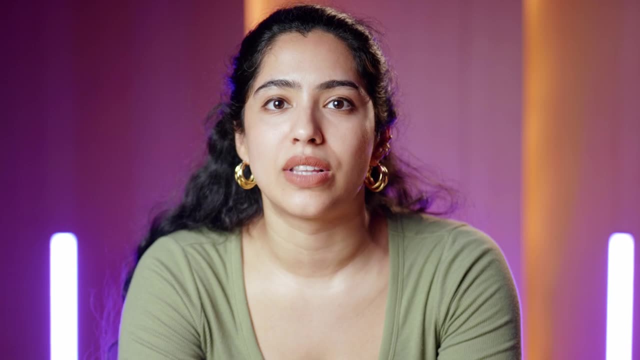 for each. First, there's the leader-follower strategy, also known as primary replica. This is probably the most common strategy, where a query writes to a single designated leader. The leader then replicates the data to a single designated leader and then replicates the data. 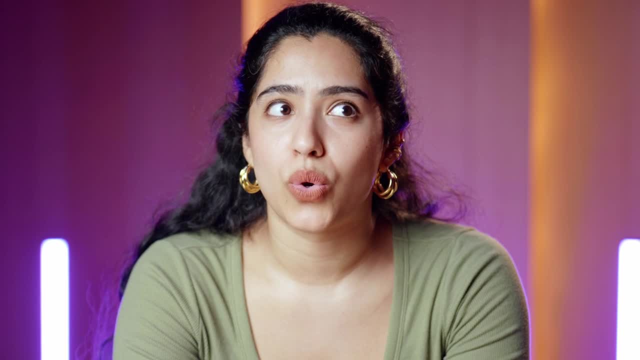 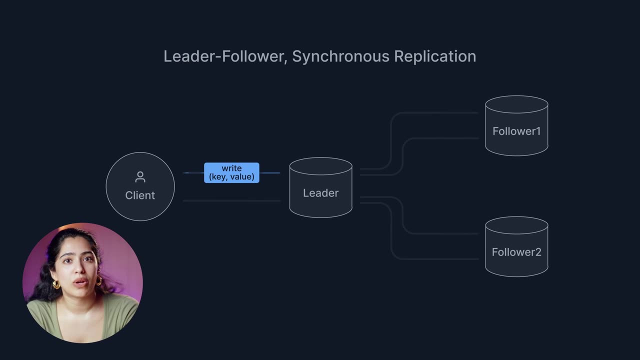 updated to followers Sounds simple enough. So what's the catch? Well, if this is done synchronously, it can be really really slow. Synchronous replication requires that both the leader and followers must commit before the write is considered successful. This does ensure that 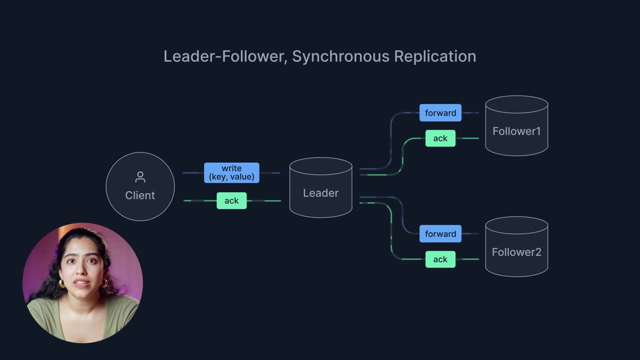 follower data is up to date, But if a follower in the chain goes down, the write query will fail. And even if the whole system is up, waiting for a follower located halfway across the world to come back up and acknowledge a successful write will raise latency considerably- Asynchronous. 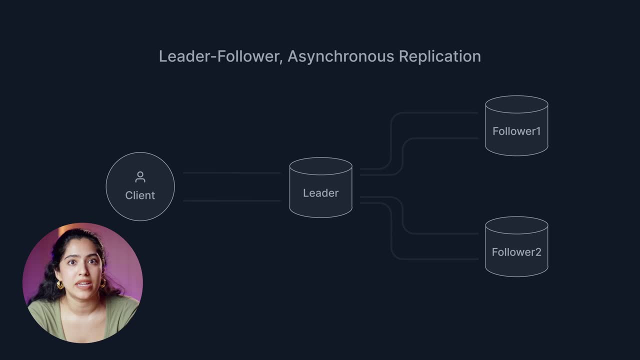 replication may be an option for use cases where transaction speed is more important than consistently accurate data. With asynchronous replication, the leader sends write requests to its followers and moves on without waiting for acknowledgement. Is this faster? Yes, But this introduces inconsistency between the leader and followers, which can be a huge problem if the 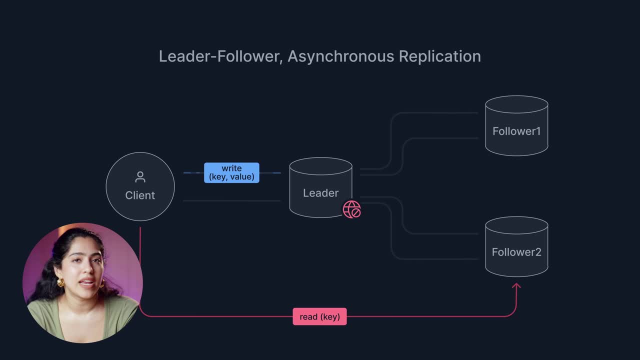 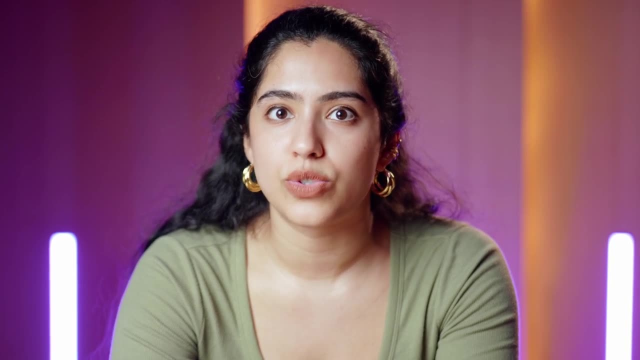 leader goes down and the most up-to-date data is lost. And make no mistake, leader failures will happen. In the case of a simple leader-follower strategy, when the leader fails, which is also called a failover, the replica is promoted to be the 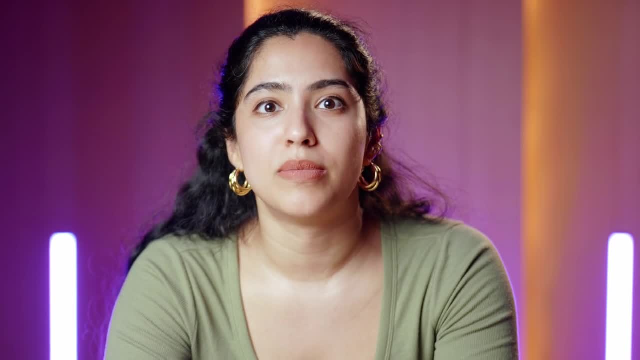 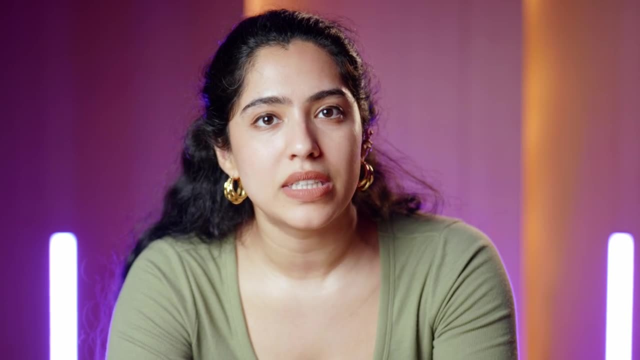 leader and takes over. Failover is a huge problem under asynchronous replication, but it's not great under synchronous replication either. Without a leader, you lose the ability to handle writes. It's absolutely critical to talk through leader failure in your system design interview. 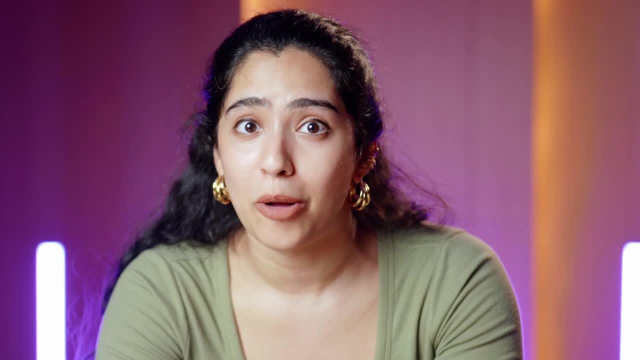 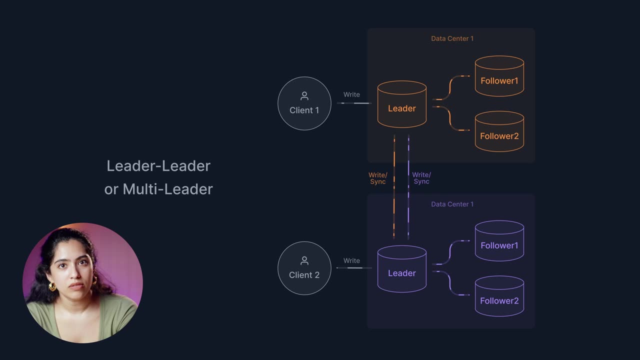 Luckily, there are a few tweaks to the leader-follower framework that can help Our next strategy tweaks leader-follower by designating more than one leader in the system. This is called leader-leader or multi-leader, and it's a simple.